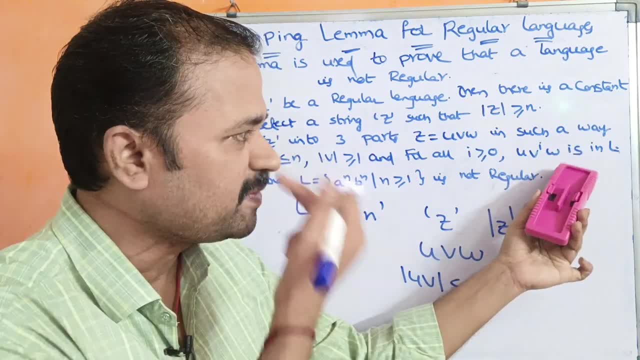 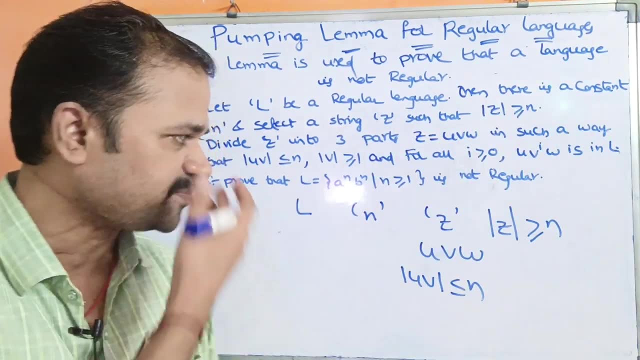 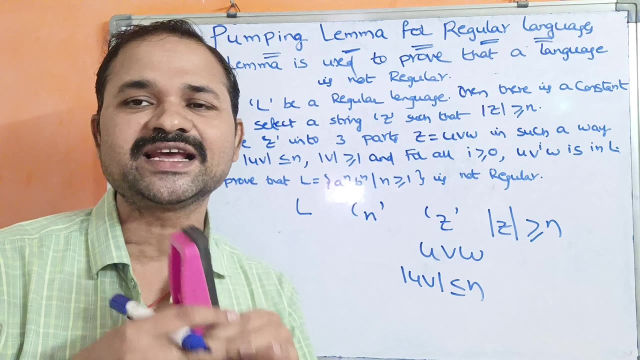 or equal to 0, u v power i, w is in L. So this is the explanation here. So let us see the explanation one more time. So L is nothing but a regular language. n is a positive integer constant. Then we have to select a string in such a way that mod z, z is nothing but. 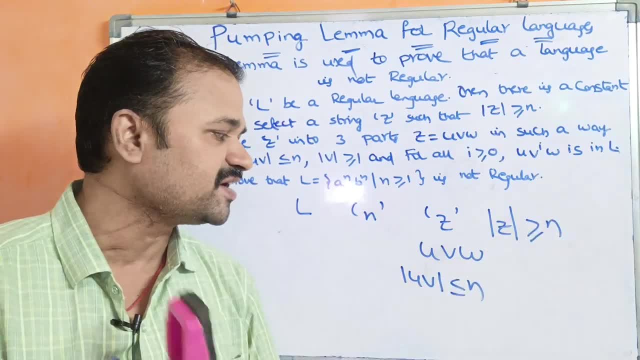 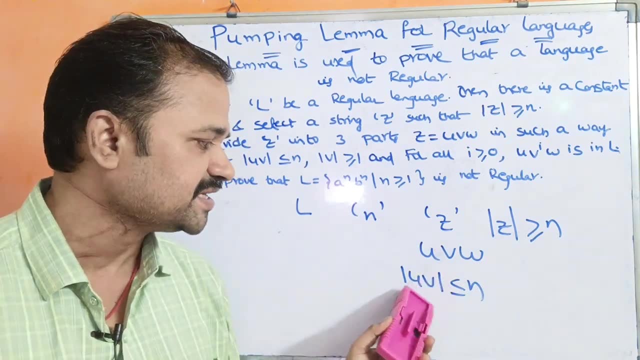 string. Mod z means length of the string. Length of the string is greater than or equal to n, Then we have to divide the string into three parts: u, v, w, such that we have two conditions. The first condition is mod u, v. 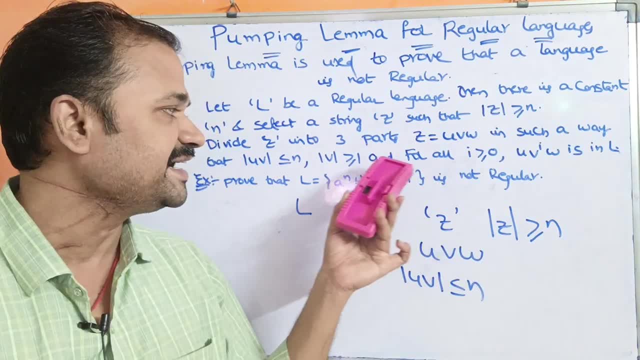 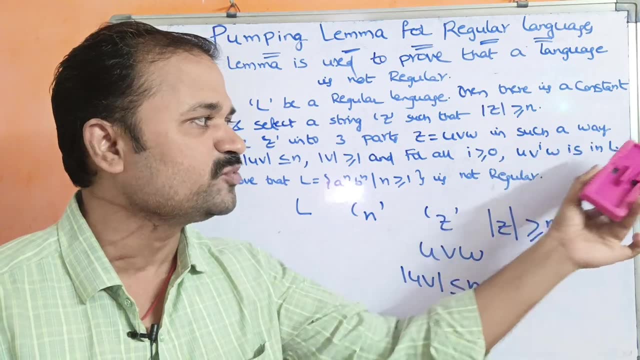 is less than or equal to 1, less than or equal to n. The second condition is: mod v is greater than or equal to 1.. For all i is greater than or equal to 0, u v power i w is in L, So let. 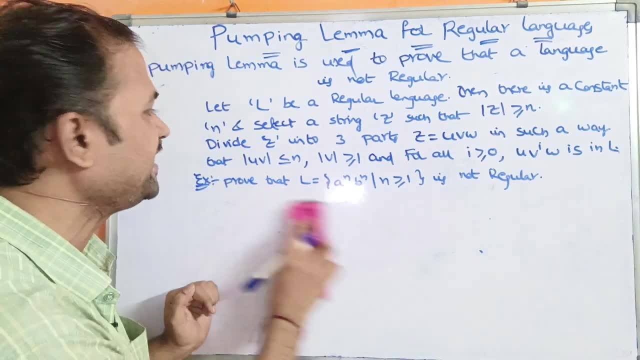 us see an example so that we will get perfect clarity about this theory. Prove that L is equal to a power, i, w. So let us see an example so that we will get perfect clarity about the world. So one can see that a power n and b power n are equal to n. So here the language. 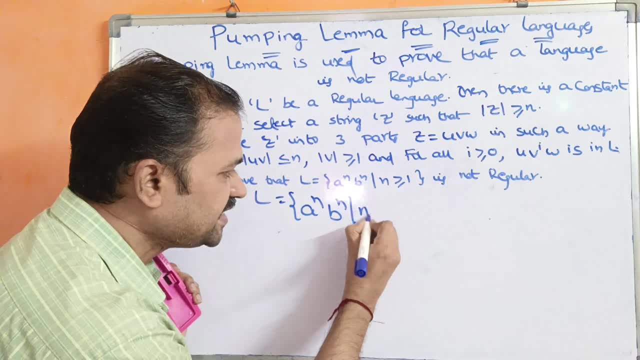 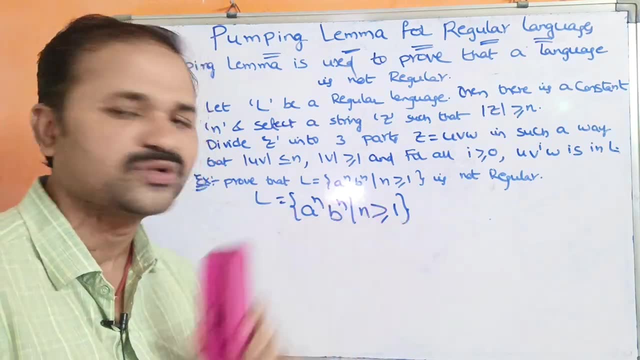 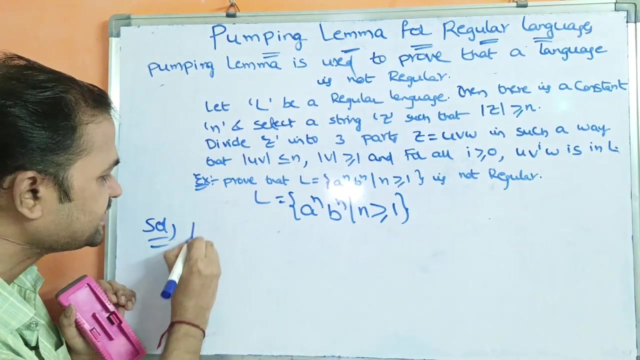 is a power n. b power n such that n greater than or equal to 1 is not a regular language. So by using pumping lemma we have to prove this language as not a regular language. So let us see the solution here. So let L is let. this language is a regular language. So 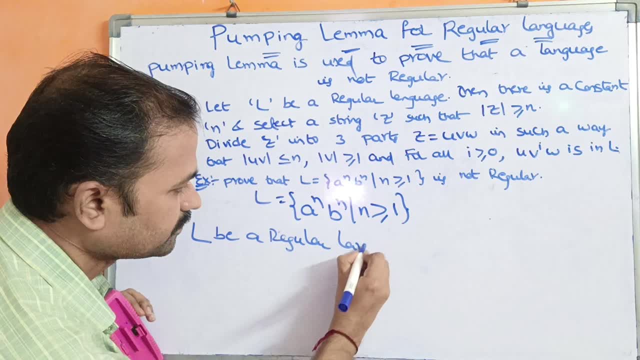 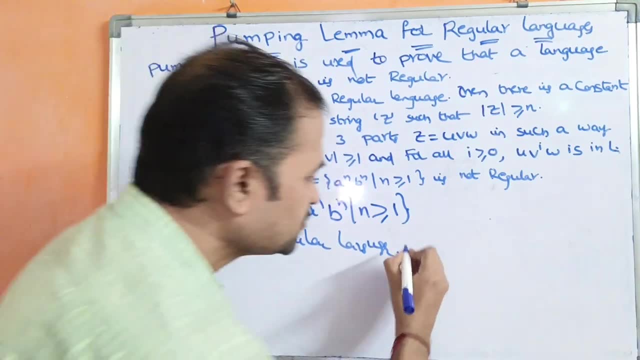 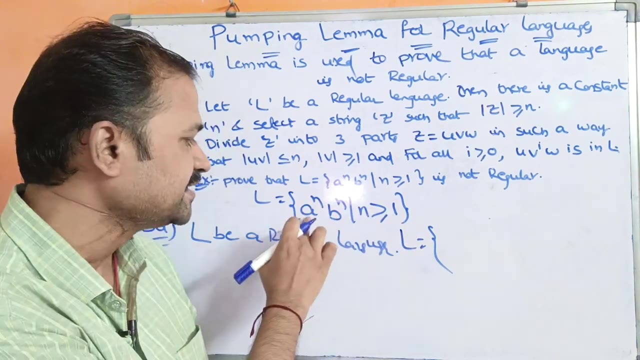 let L be a regular language. there is a constant n, So we have to assume some constant. So before that, let us see the strings here: n, greater than or equal to 1.. If n is equal to 1, then what is the language? a power 1, b. 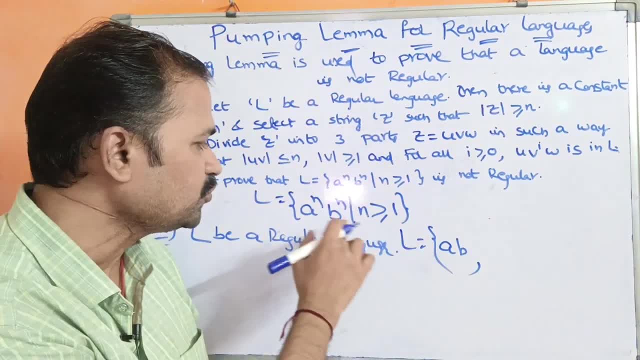 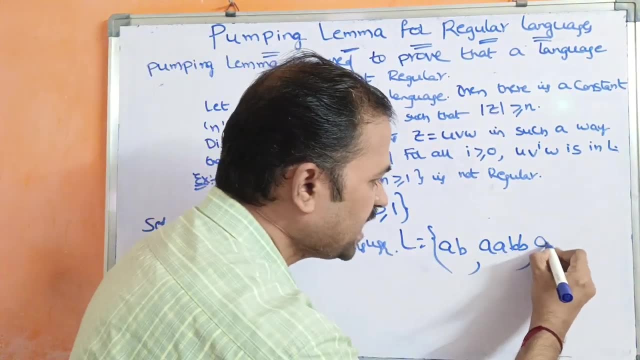 power 1. That is nothing but a- b. If n is equal to 2, then a power 2,, b power 2. That can be written as a a, b, b. If n is equal to 3, then a power 3.. So 3 a's, 3 b's, So on. So likewise we can have 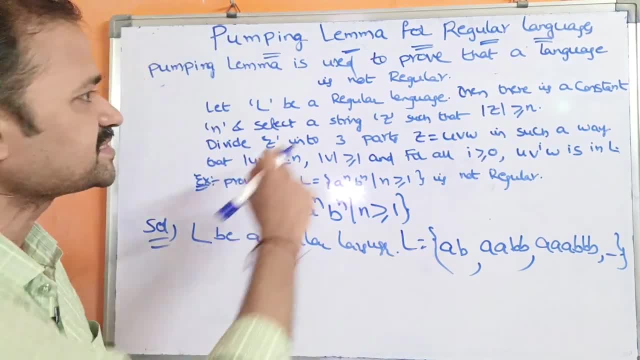 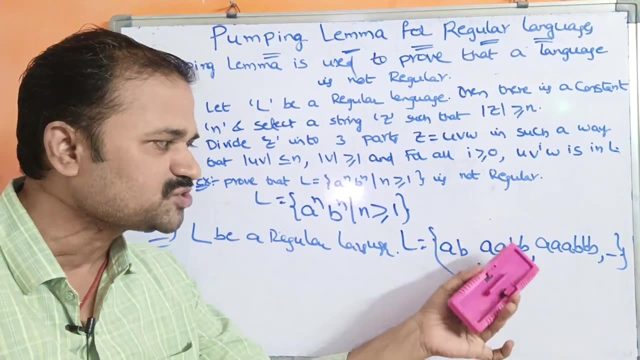 n number of strings in the language. So this is the language. Then there is a constant n. Now we have to assume n value. So it is our choice. We can assume n? ya's 2, n ya's 4, n ya's 6 or n ya's. 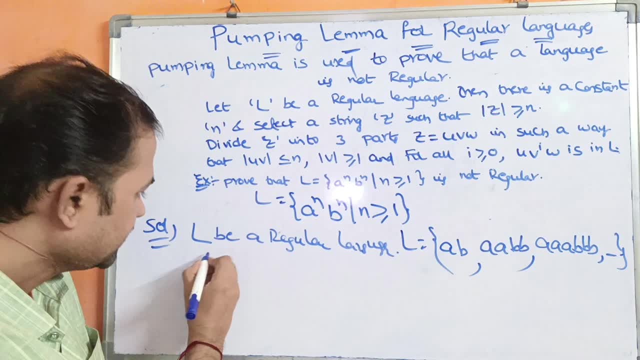 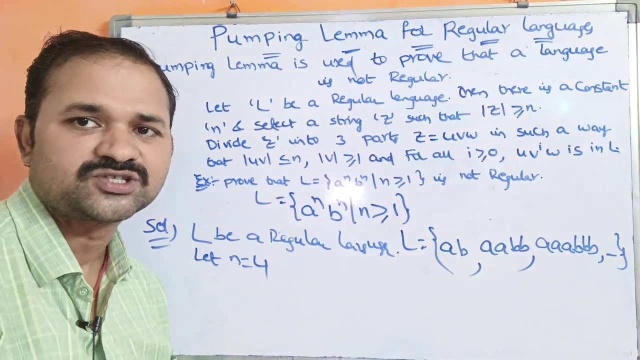 8. We can assume any value. Okay, So let n is equal to 4.. Let n is equal to 4.. Okay, So that means we can take: the length of the string is 4 characters. Okay, Let n is equal to 4.. Okay. 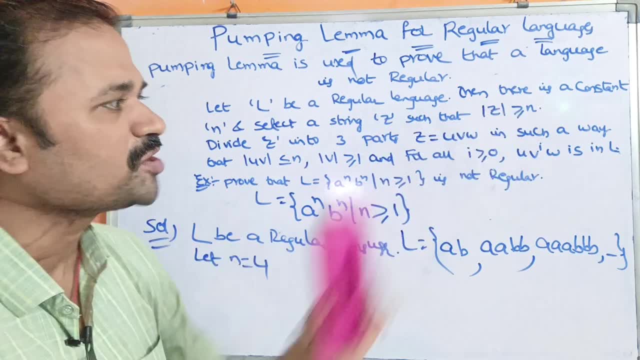 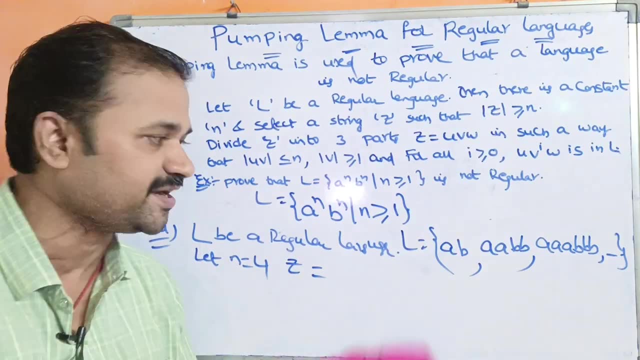 So n is equal to 4, and select a string such that mod z is greater than or equal to 1.. So we have to select a string in such a way that mod z is greater than or equal to n. So let g is, let z is. 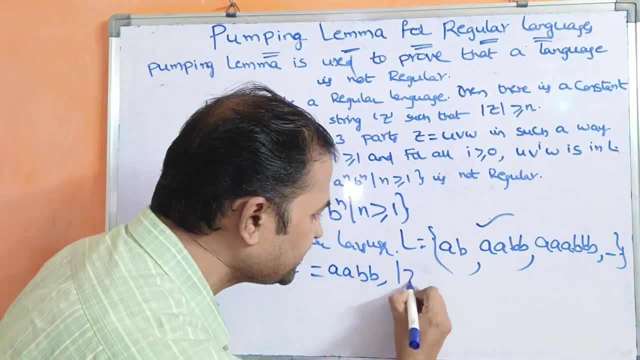 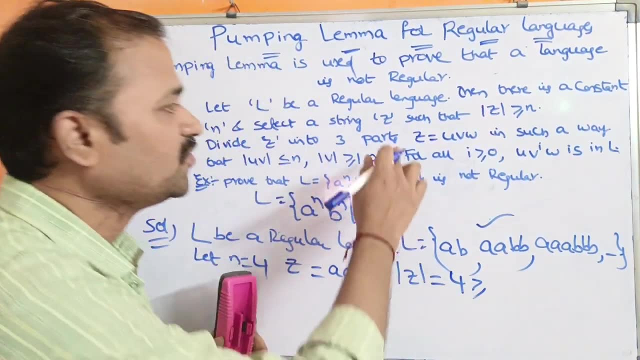 equal to a, a, b, b. Then what is mod z? So mod z is equal to. mod z means length of the string 4.. So 4 is greater than or equal to. what is the condition? Mod z is greater than or equal to n. 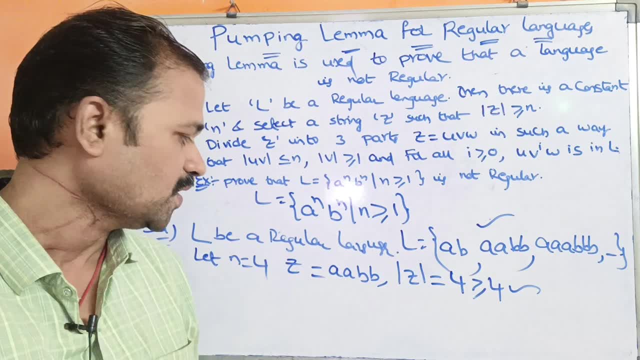 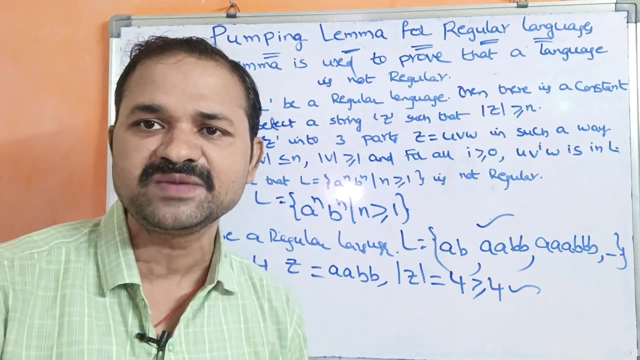 So 4 is greater than or equal to 4.. Condition is true, Or we can assume the string ya's 3 bull a, 3 bull b. Then what is the length of the string? 3 bull a means 3 characters, 3 bull means 3 characters. 3 plus 3 means 6.. So 6 is greater than or equal to. 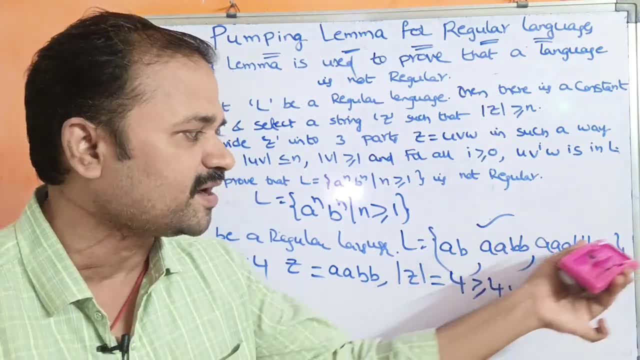 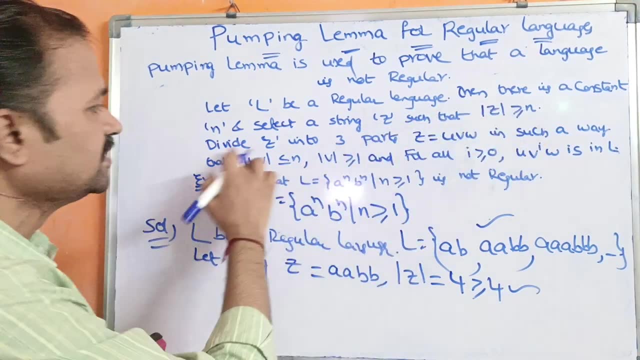 4. Condition is true. So we can assume either a a, b b or 3 bull a, 3 bull b. So likewise we can assume 4 ya's, 4 b also. So that is our choice. So this is over. Next divide z into 3 parts. 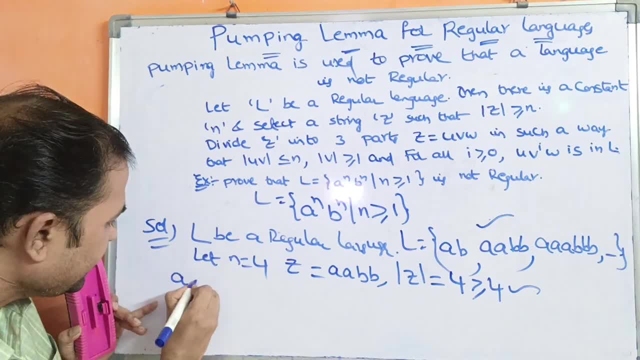 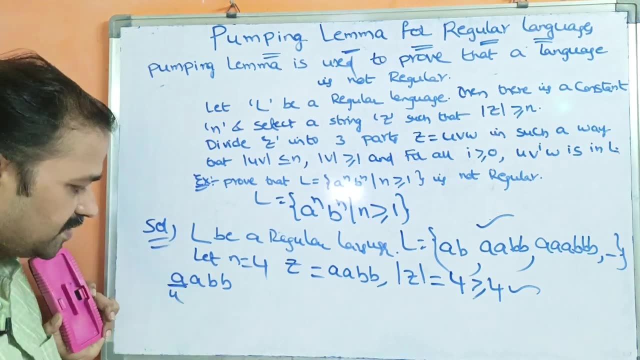 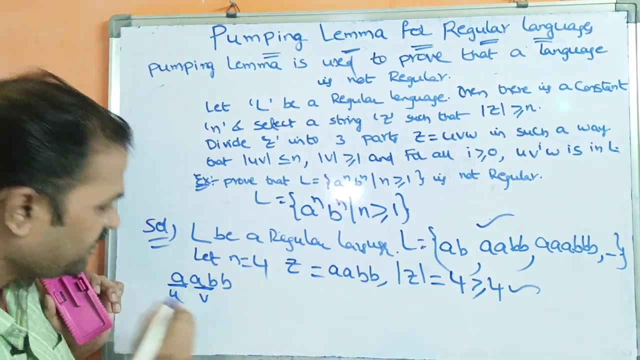 u, v, w Here. what is the string? a, a, b, b is the string. Divide the string into 3 parts. Let us assume that this is u. It is our choice. Let us assume that v means a, b, w means b. So here we are, dividing the string into 3 parts. 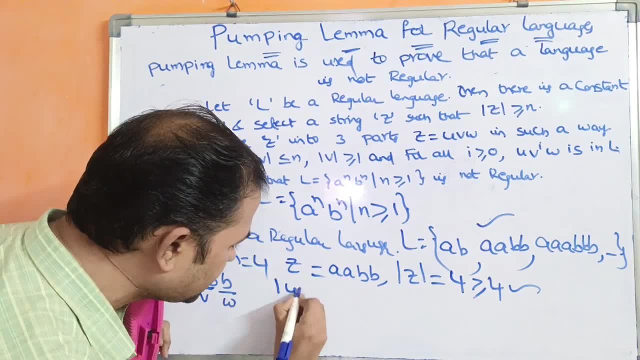 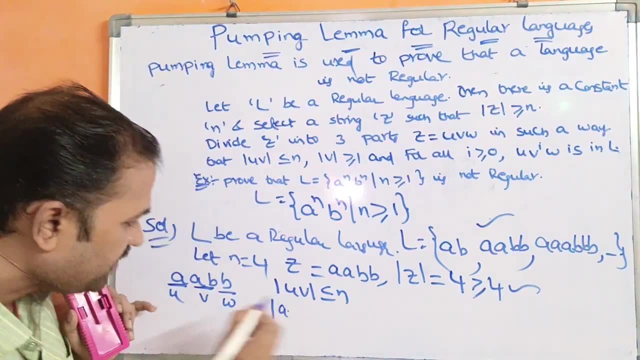 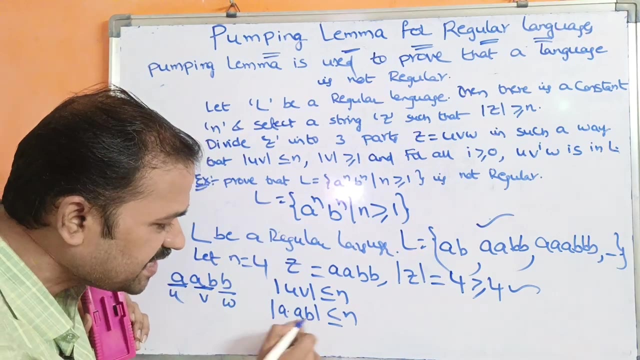 Such that what is the first condition? The first condition is: mod u, v is less than or equal to n. So here mod, what is u, u means a and what is v, v means a, b is less than or equal to n. So mod a, a, b means here we have 3 characters, So 3 is less. 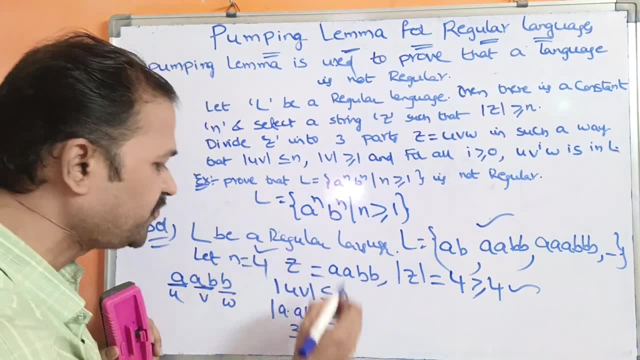 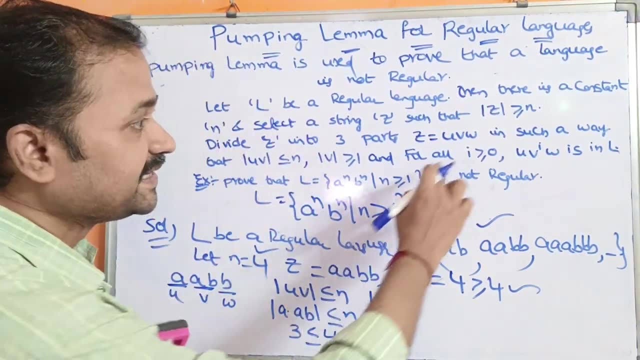 than or equal to what is n? In this problem, n value is 4.. So 3 is less than or equal to 4. Condition is true. And what is the second condition? Mod v is greater than or equal to 1.. 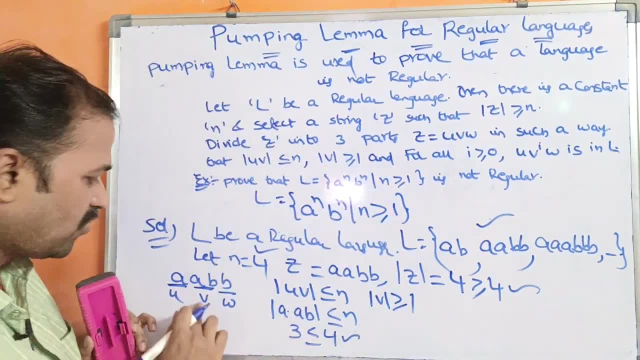 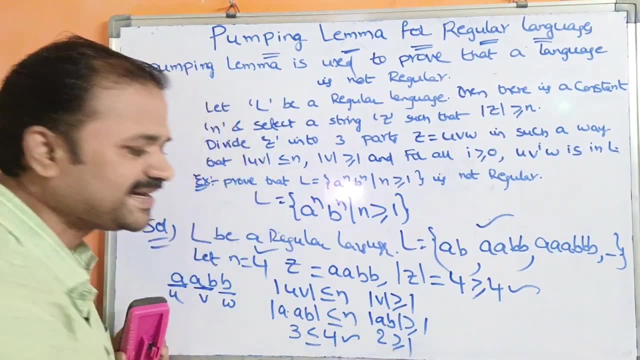 What is the second condition? Mod v is greater than or equal to 1.. What is v here? a, b. So mod a, b is greater than or equal to 1.. So a b has 2 characters. So a b is greater than or equal to 1. Condition is true. And we have one more condition. 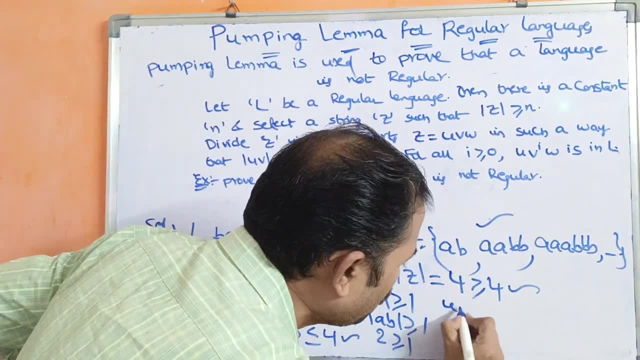 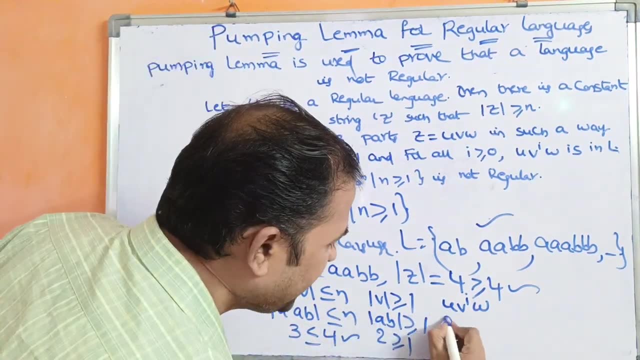 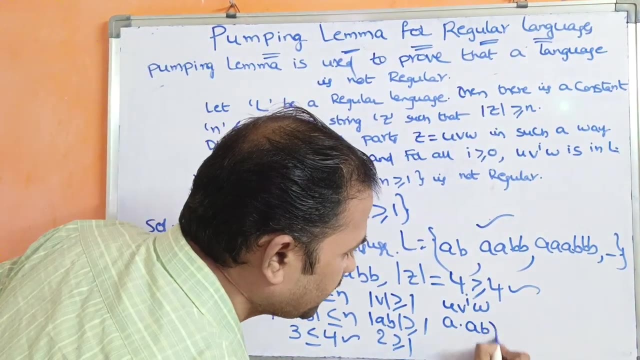 For all i greater than or equal to 0, u, v, power, i w is in n. So what is u here? u means a. What is v here? a power, b, a, b. b means a, b, a, b, whole power, 0.. What is w, w means b, w, b. 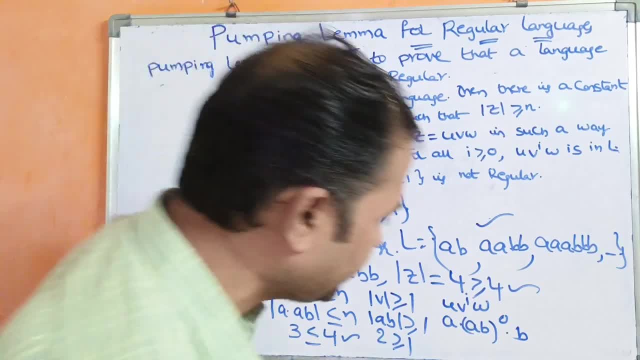 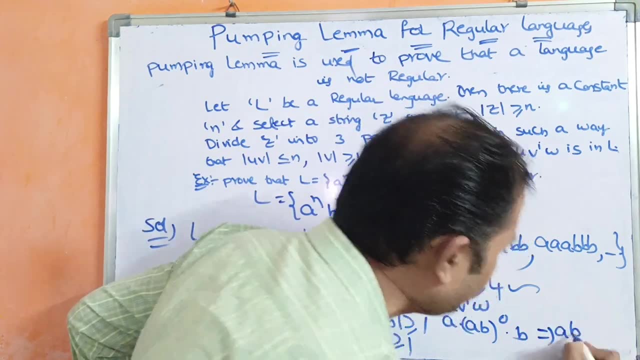 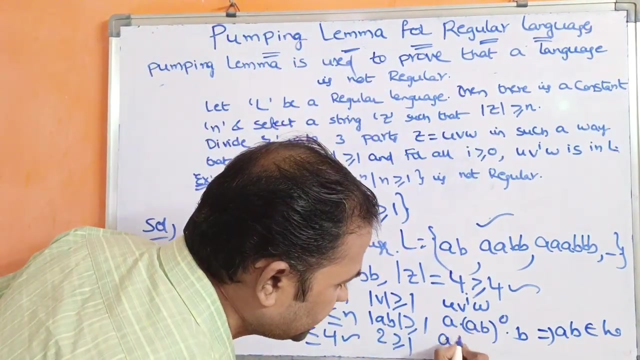 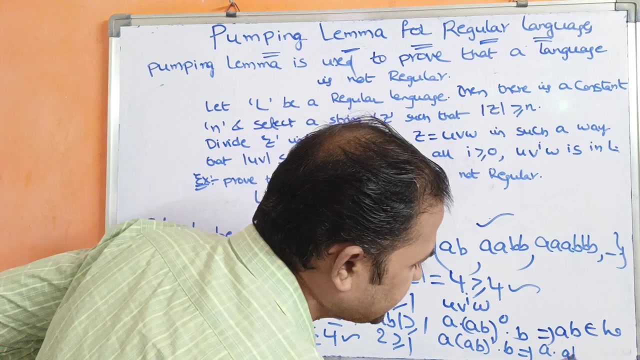 w. This total ANDUNG value of a. w requires 1 here as its capital. This partially functions under a thing, but simply means it is performlands only. For a visual value of b we have 12 put 1,. 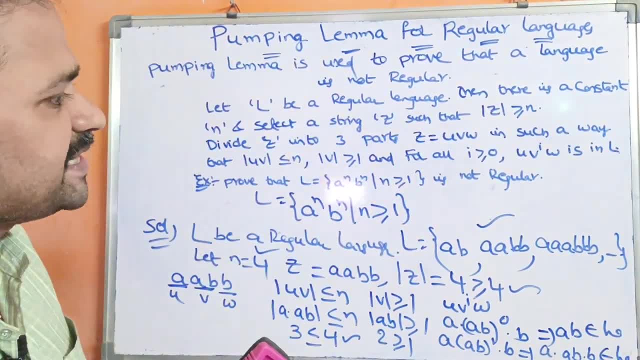 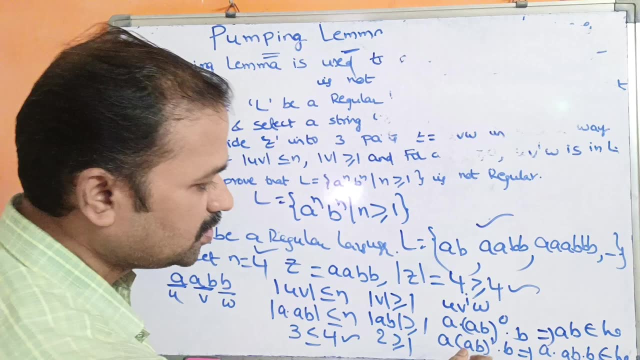 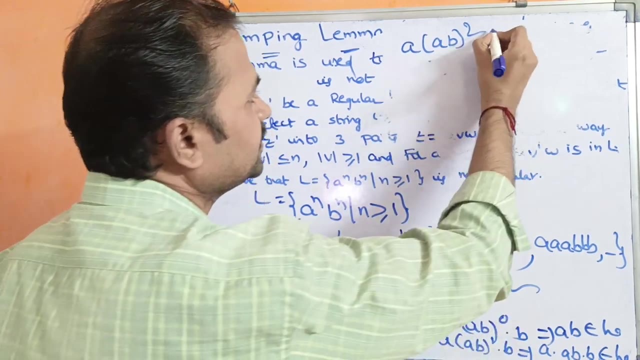 in the language. So belongs to n, So for space constraints, let us erase this portion. Let us erase this portion Now. let us assume that i is equal to 2. So then we can write as a into ab, whole power 2 into b. So this can be written as a into ab. whole power 2 means 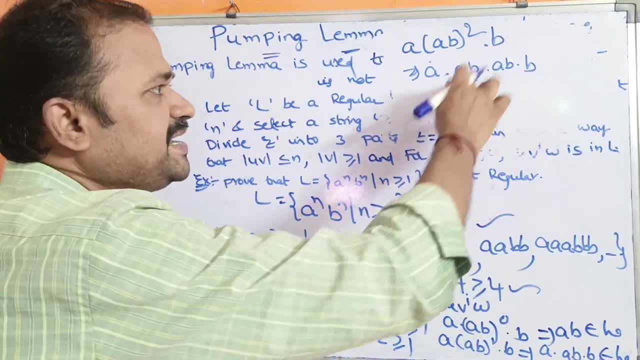 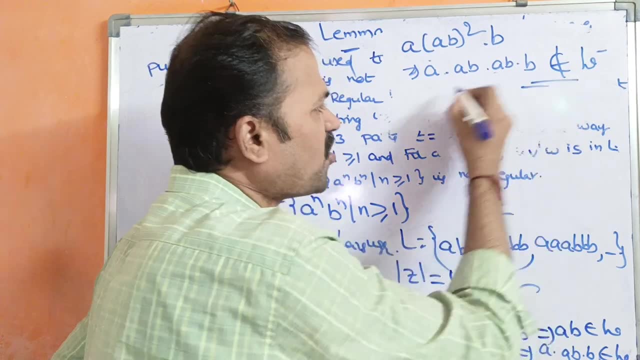 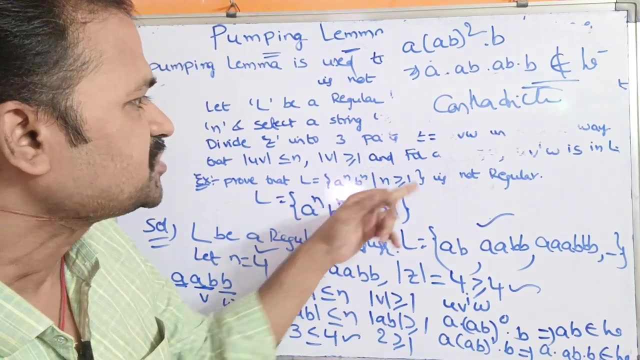 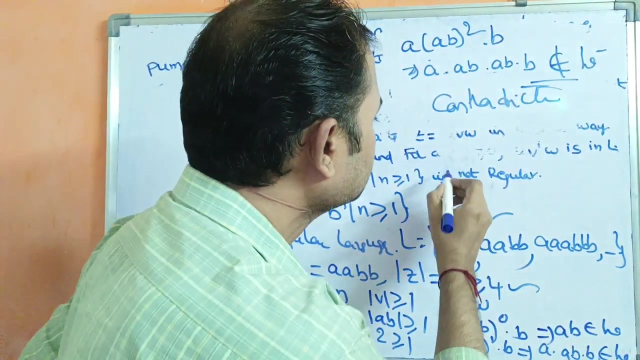 ab into ab into b. So double a b a b b. So double a b a b b. So this is not present in the language. So this is contradiction, Contradiction, Contradiction. Initially we assumed that, we assumed that and for for here. what is the condition For all? for all, for all v greater. 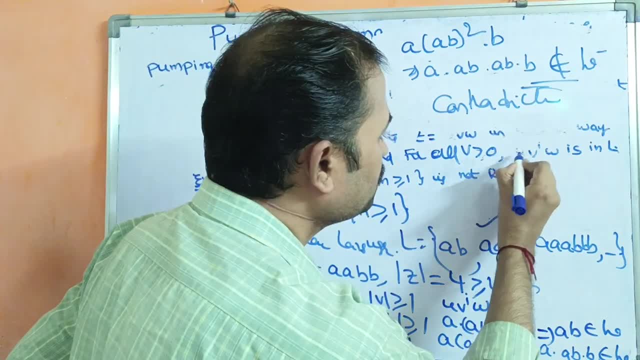 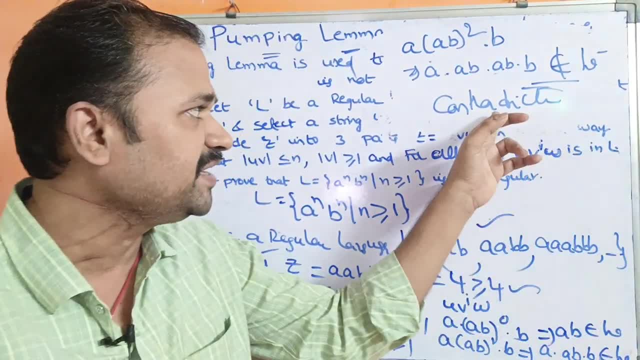 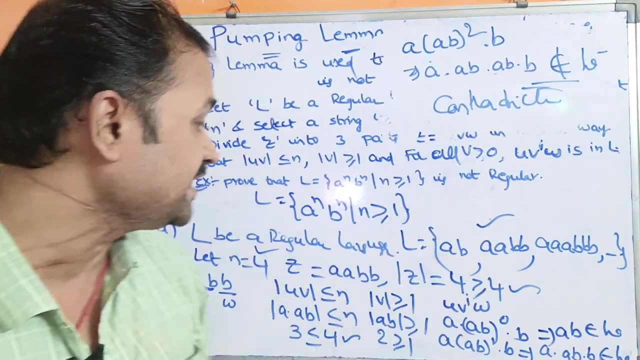 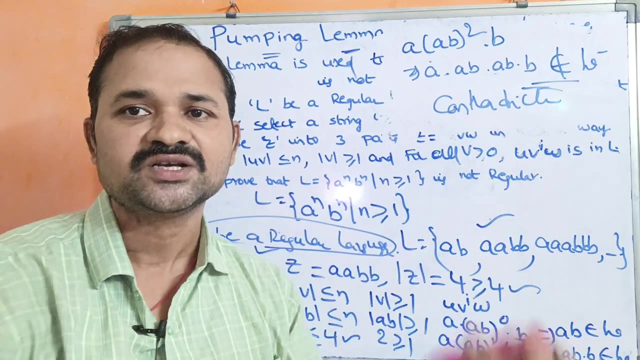 means this string must present in l, But here we proved this, as this string is not present in the language. So this is the contradiction. So we can: initially we assumed l as regular language, But now prove we proved the contradiction, So opposite. So we can say that this language 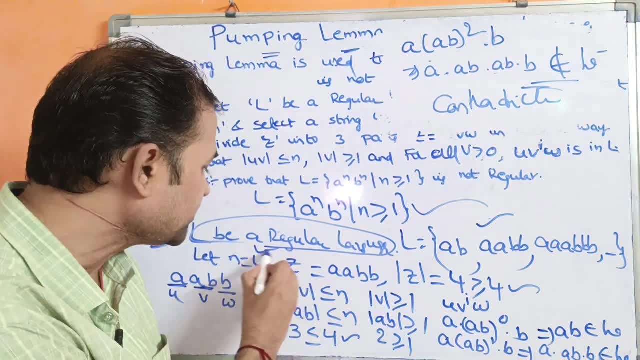 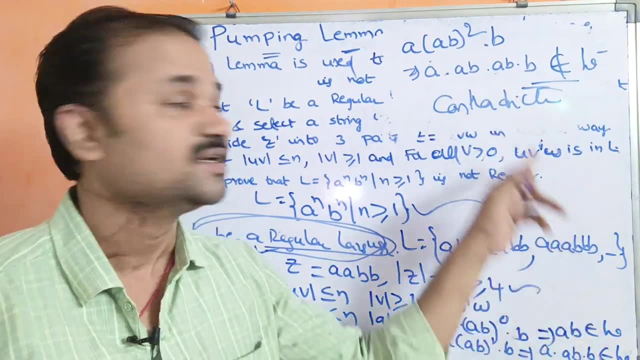 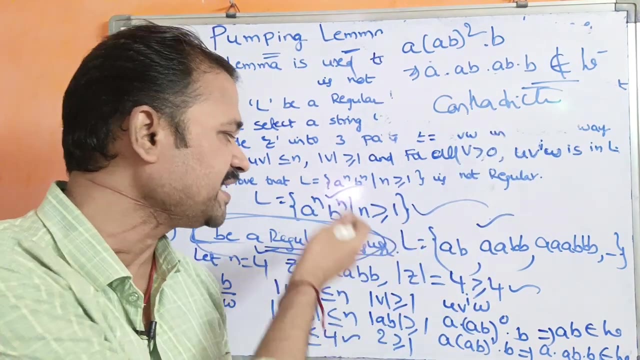 is not a regular language. Why? because initially we assumed this as L as regular language, but here we got a string which is not present in the language. So this is nothing but contraction, So opposite to the assumption. So we can say that L is equal to a power n, b power n such that n greater than or equal to 1. 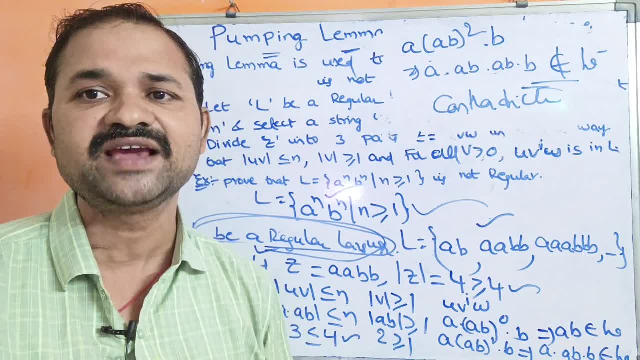 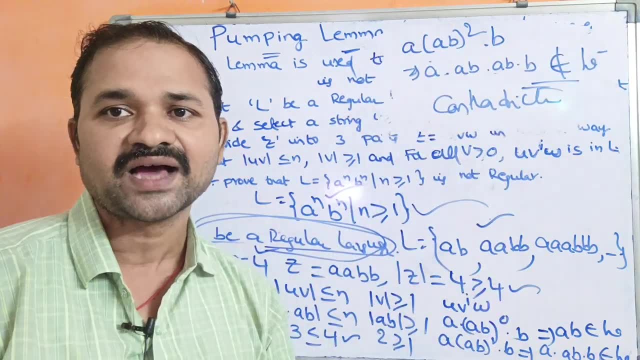 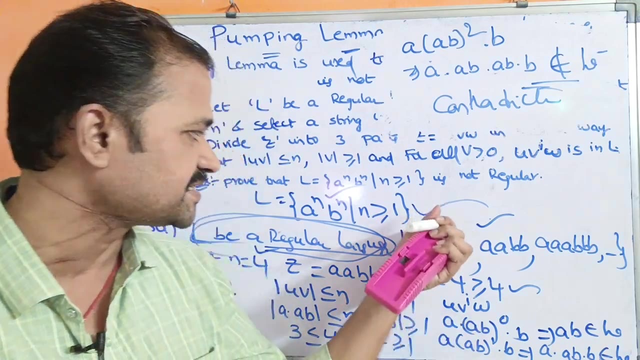 is not a regular language. So likewise we have to prove that. Suppose, if this string is also present in the language, then we have to assume I as 3.. I as 3, let that string is not present in the language, So that is called action. So we can say that this language is not regular language. 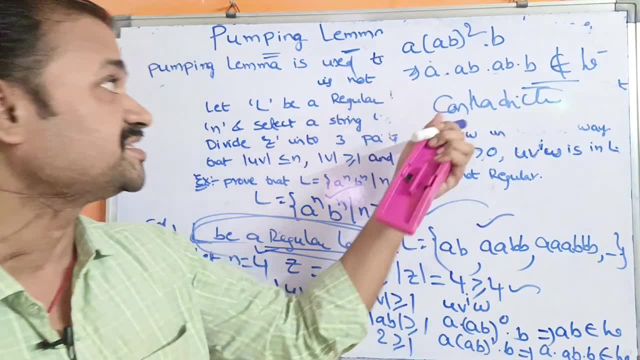 So in this way we can prove a language as not regular: by using with pumping lemma.